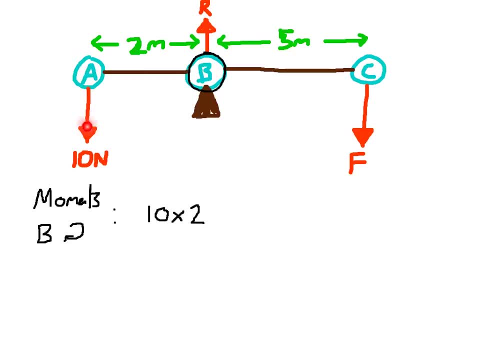 B is the centre of my clock. So this force of 10 newtons, if you consider it, would go round anticlockwise. So that means it is negative. I write negative. The next force I need to consider is this: R newtons here. 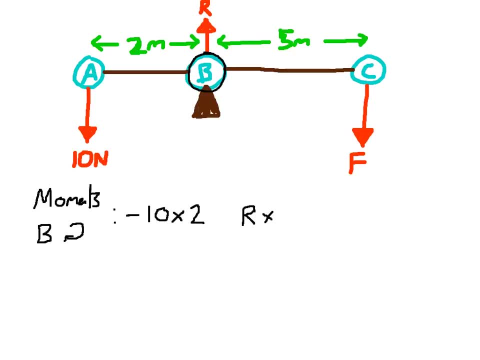 But you'll notice the distance from the centre of my clock from B to R. well, it's 0. So in fact that doesn't have any effect on the equation. The final force is F over here. So I need to take F times the distance from where I'm taking moments, and that's 5.. 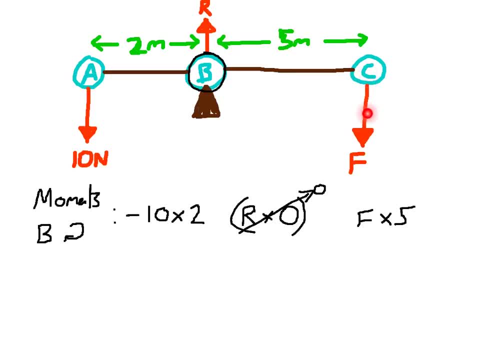 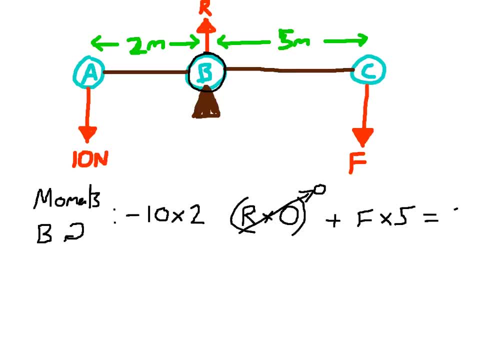 up are not having any turning effect and therefore equal 0. We can very quickly solve this: Minus 20 plus 5F must equal 0. So quite clearly then, F would have to equal. take the 20.. 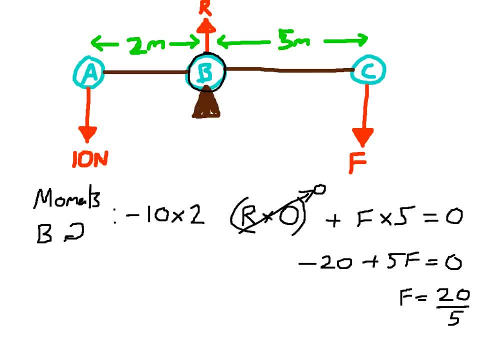 Take the 20 across and divide by the 5.. F equals 4. And that's the answer to this question. I haven't found R because taking moments at B meant the distance to R was 0. Now I could have found R by taking moments at a different point. 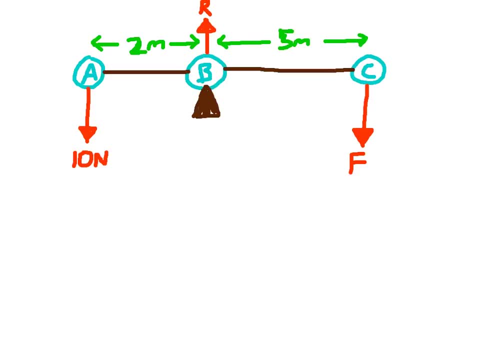 For example, I could take moments at C. Let's now take moments at the point C and see if that helps me find R. So tell the exact examiner you're taking moments. I'm going to take them at C this time and I'll still take them clockwise. 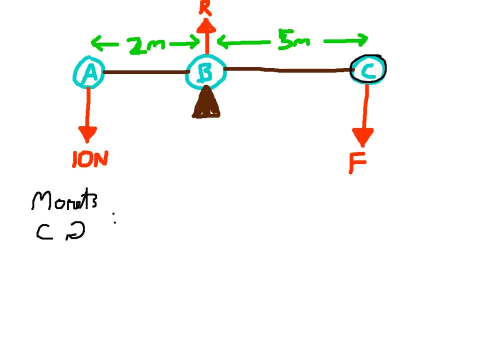 I always do clockwise, regardless of the context of the question. So the first force to consider is the 10 Newtons. So I take the 10, and I times by the distance from where I'm taking moments to that force. You can see that as a distance of 7..